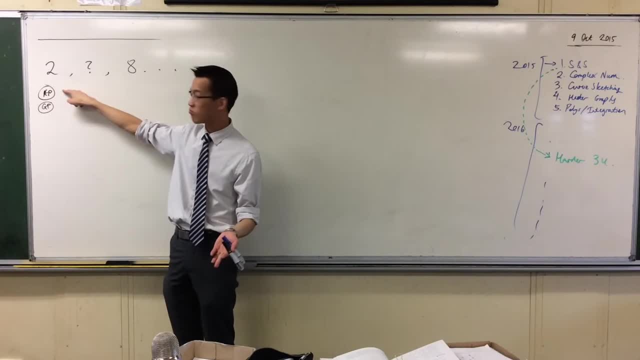 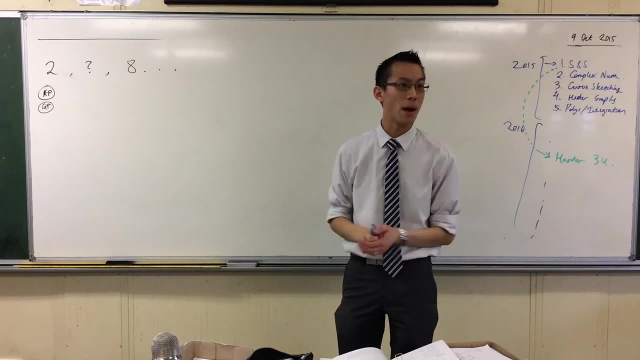 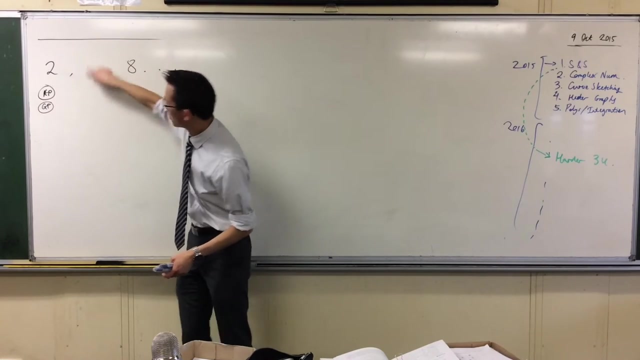 I can make this sequence an AP or, if I want, I could make it a GP, depending on what number I put in there, right? Because since I don't know yet, it's still up to chance Now I've chosen really small numbers. What number would I put in here to make this an AP? 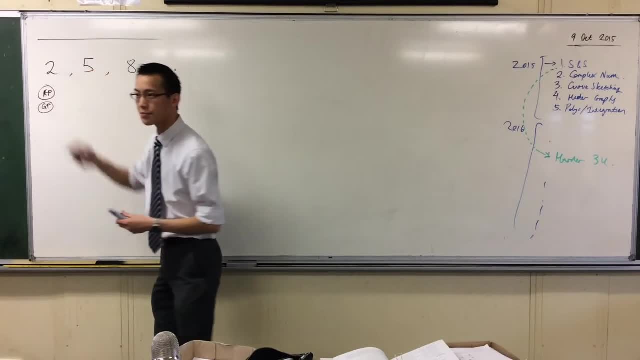 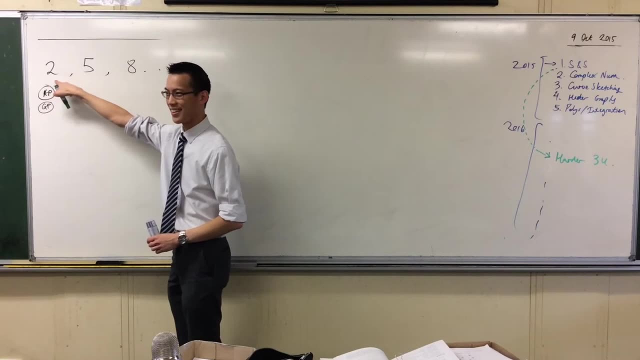 I would put five. How did you get five? Because you take the first one and you subtract the third term and because you know that there's a common difference between the first and second and third and fourth term. so the common difference is twice if you jump from the first term to the third term. 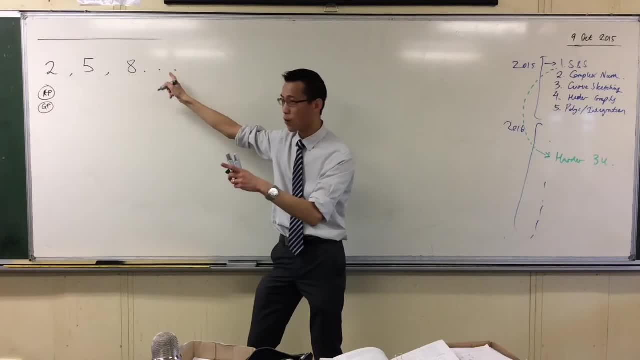 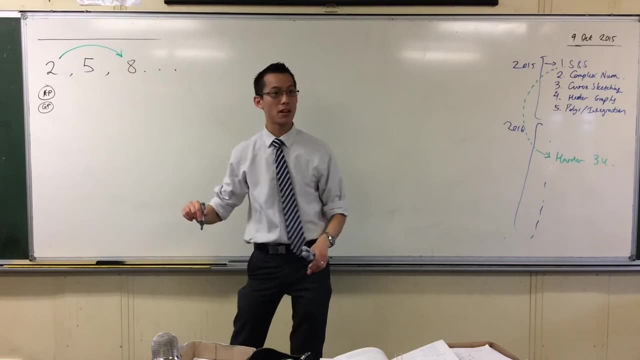 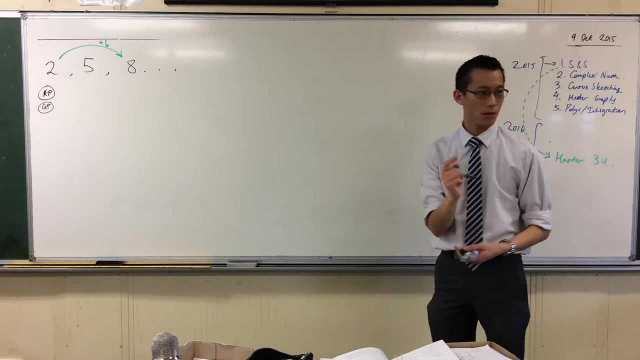 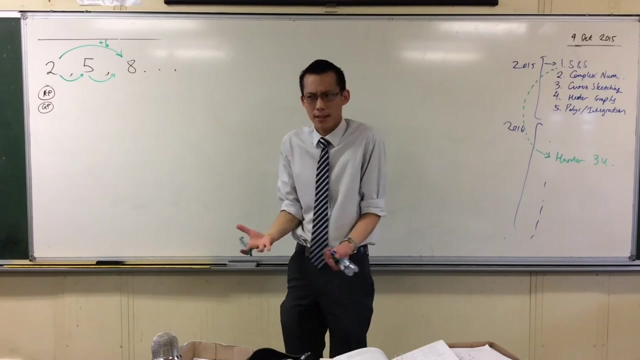 Sure, Okay, good, I think I followed that, but somehow a fourth term snuck in, which is fine, Let me see. if I understand, and you guys follow with me, We have a little Look at this gap, This gap here, and the gap is six Plus six. If there is one number intervening between those, that means that plus six really represents two steps of plus three plus three. That makes sense, doesn't it? 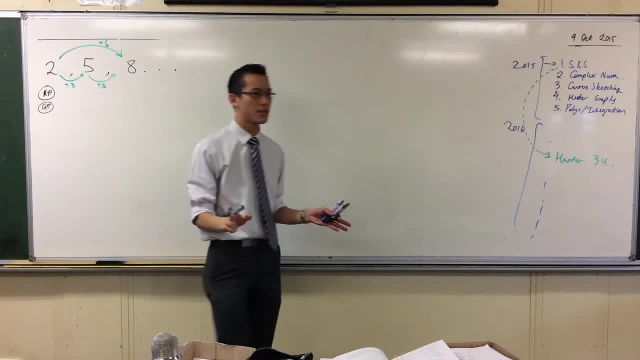 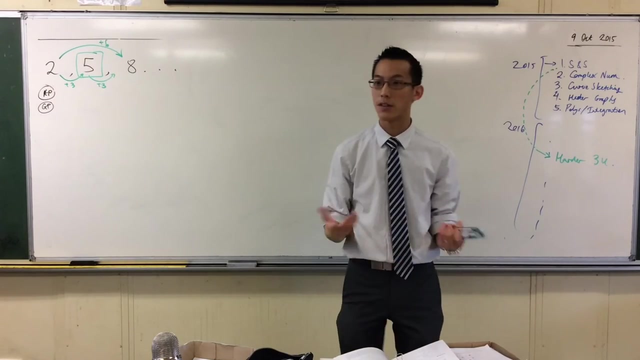 Okay, so plus three, plus three, Okay, that's fine. alright, Let's think about it another way. okay, This number five. it has an important relationship with the numbers two and eight. right, It's not just a random number, The number five. like I couldn't have just done this, Instead of taking the difference, I could have added these two, two plus eight, and to get to five, I would divide by two. 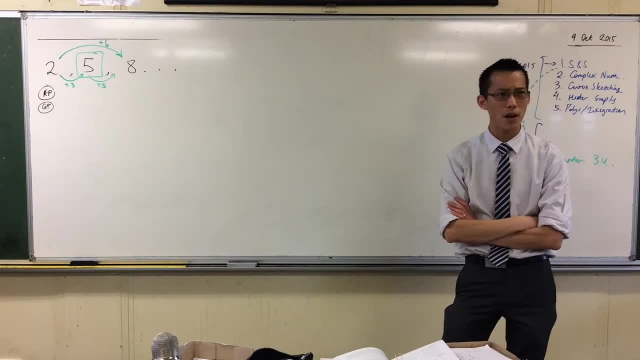 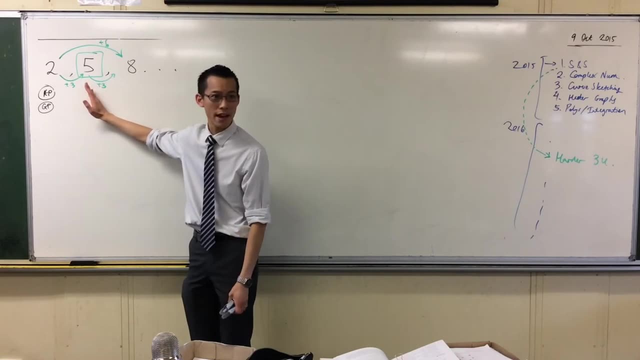 Why would I? Why does that work? Why does that give me the number that I want? It's the average, isn't it right? It's like I want. the Another word for average in our context is midpoint right, And we know exactly what the midpoint formula looks like. It's, you know, x1 plus x2 on two, and the y's as well. 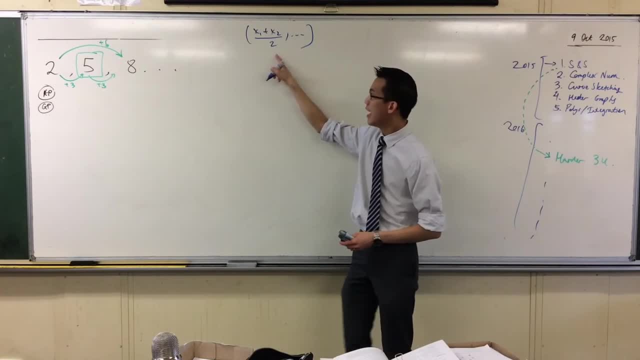 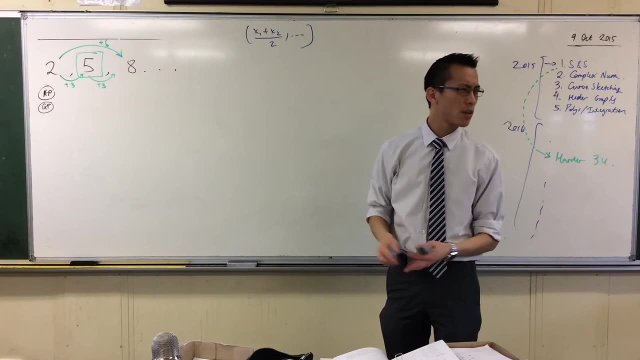 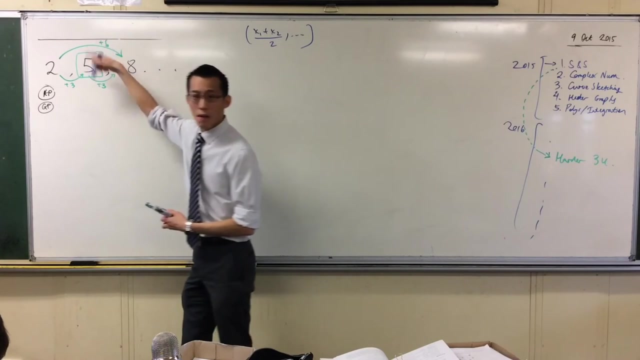 Okay. so if you want to get somewhere right, bang in the middle and you're going by pluses, you'll take the average. okay, That's fine, okay, Well, by the way, we have another word for average, a more technical one, starting with an M Mean. right, Okay, now let's label this. Five is the mean of two and eight. It's the mean of two and eight, but it's the particular mean that makes it an arithmetic progression. so I'm going to be a little more fine and call this the arithmetic mean. 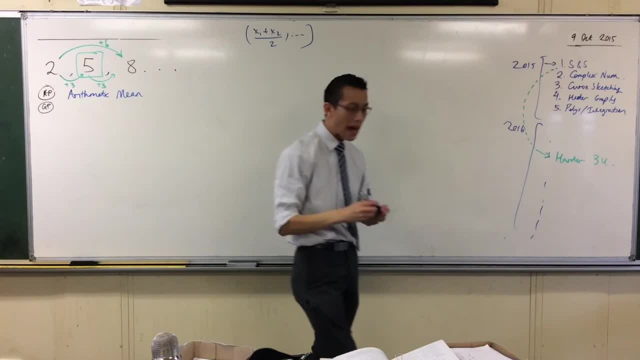 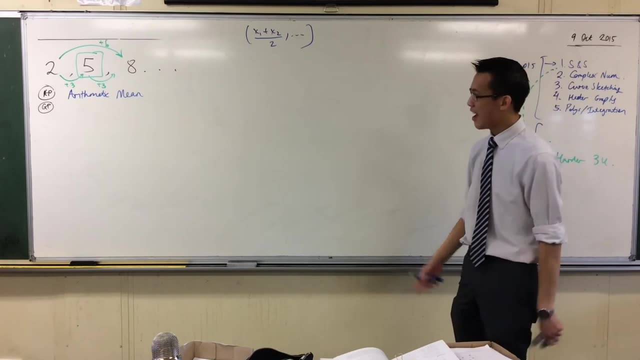 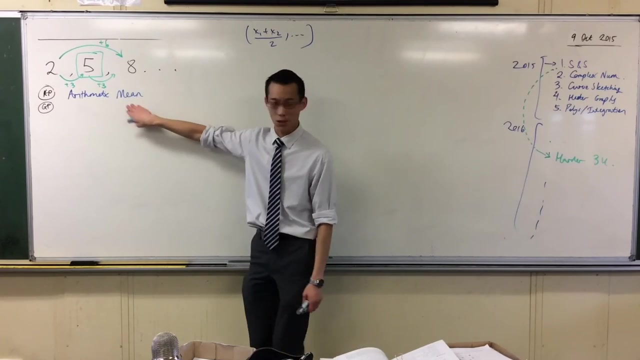 Okay now. you've never had to qualify the word mean before with an adjective, because you haven't known about any other mean. That's the only kind that there is. In fact, there are many, many different kinds of means. I'll tell you about at least two more today, but one more is important to us. 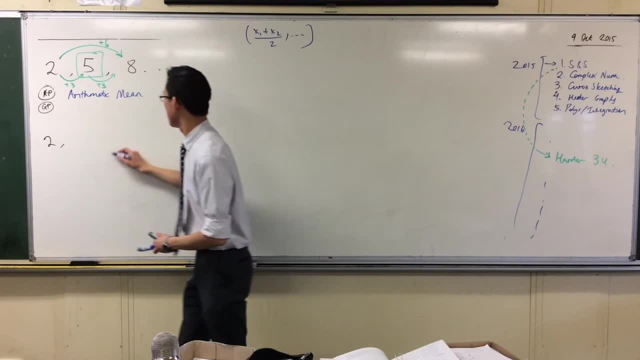 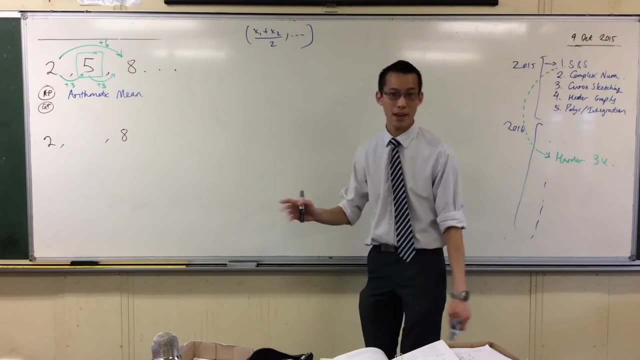 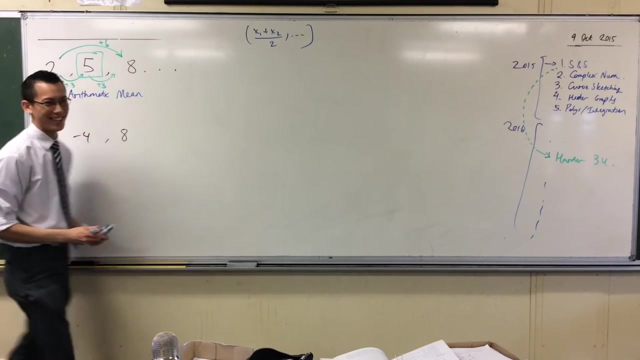 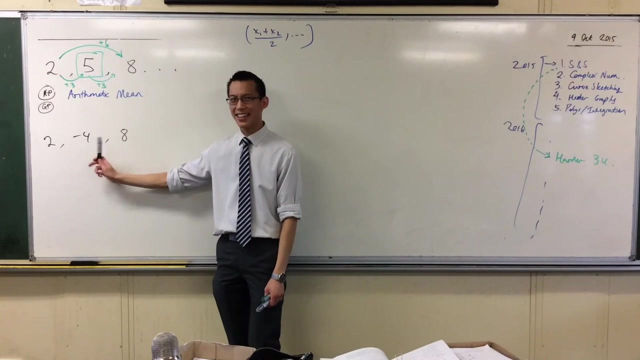 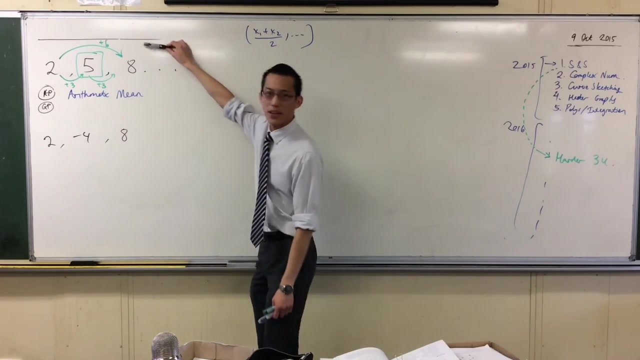 Let me write these sequence of numbers again: Two and then something, and then eight. Now I want to think geometric. okay, What number could I pop in the middle there? in order to make this a general? I could put minus four, okay. So let's have a look at this for a second. How did someone's brain contort to get that? And it's fine. okay, Let's try and make a comparison to what we did up here. You see what we did here. 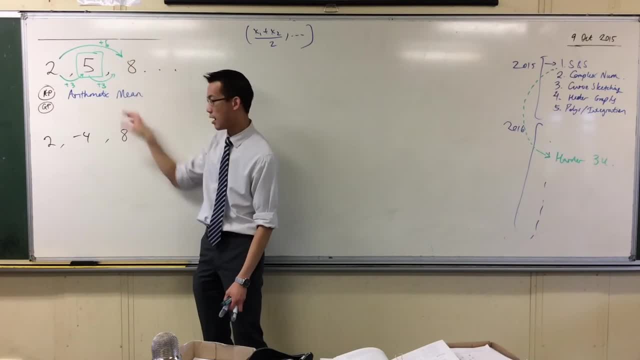 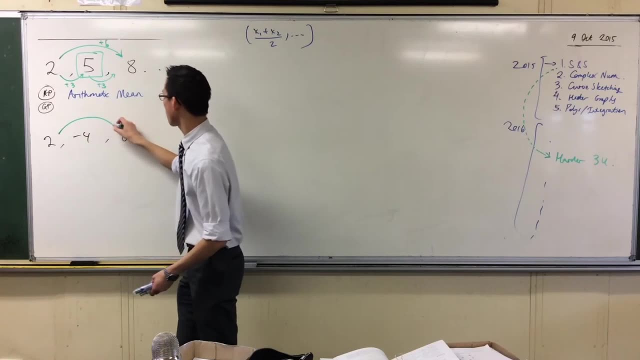 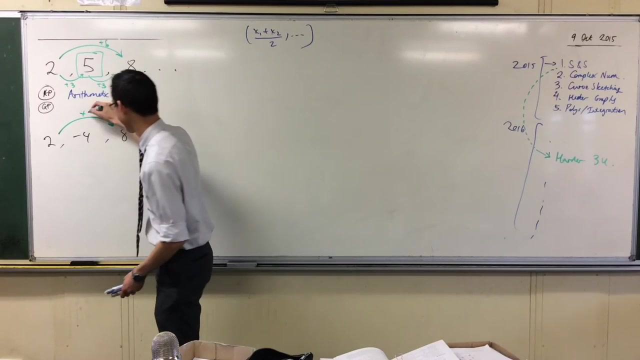 So, instead of thinking about what would I add, I'm in GP mode, right. So I'm going to need to think about what I would multiply by, because that's what makes it a general, That's what makes it a GP, right. So I went from here to here. that's two steps, and I'm multiplying by four, right, To get from two to eight. 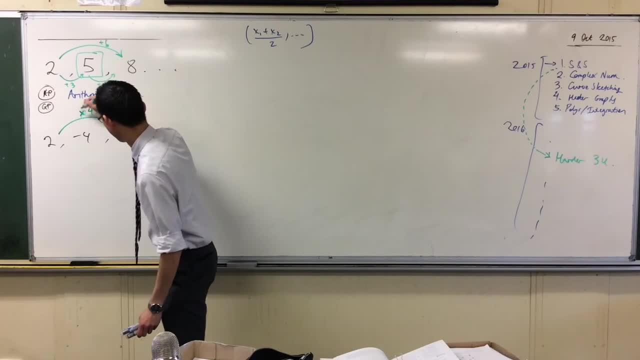 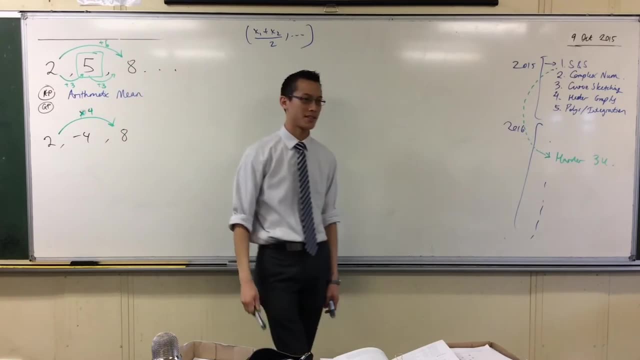 That was the next thing I was going to say. okay, So I should write my time, so it's really clear. okay, So now I just need to think about, just like: if I do plus three plus three, I'll have plus six. What multiplication can I do twice in order to get four? 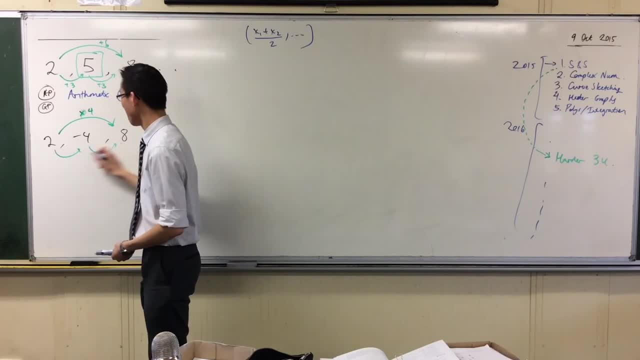 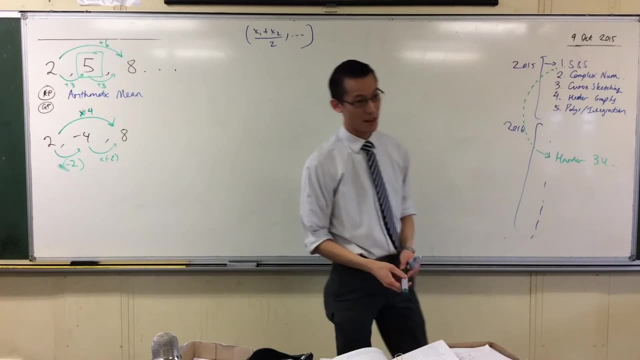 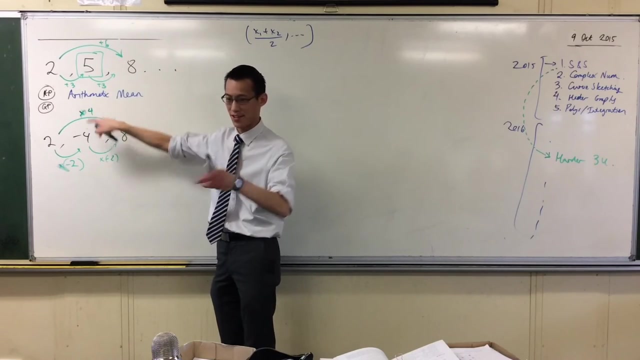 And, of course, if you're Brendan, you say: well, Sorry, times negative two, times negative two. that'll get me there. And sure enough, it will okay, Because if you say I've got a number and if I square it I'll get four, there are two solutions. 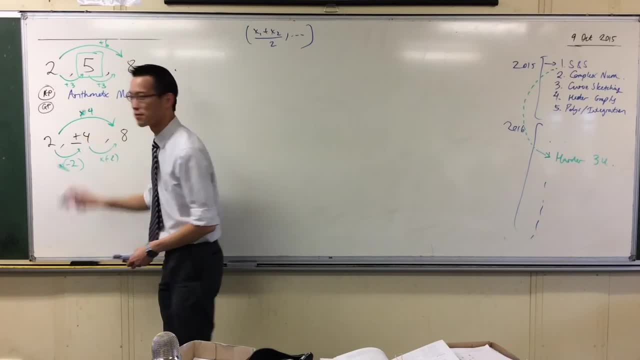 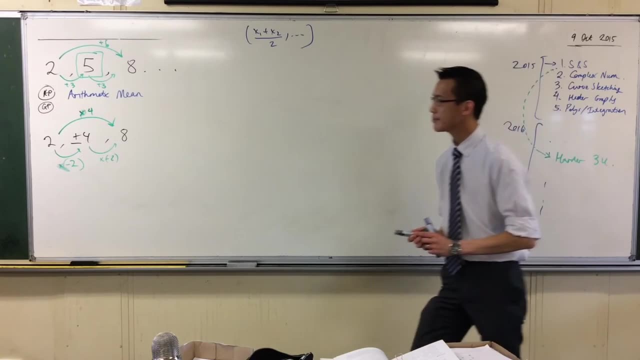 So let's be, let's be a little more accurate now and say: this is really plus or minus? okay, I could put either of those numbers in and sure enough, I would get a GP. okay, Now this, this is a number that, in a real sense, is still in the middle. 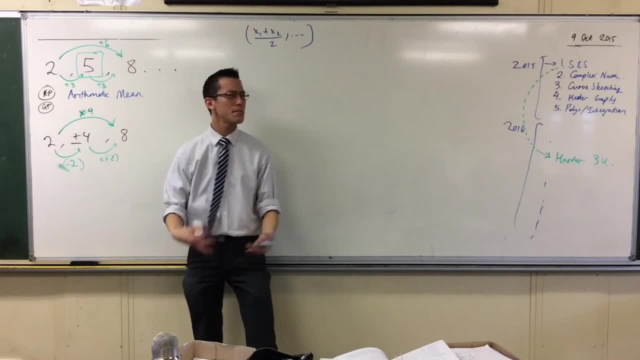 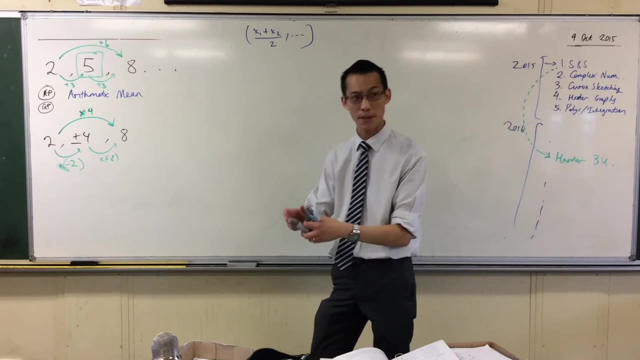 Middle, inverted commas, of these two numbers. It's just in the middle, in a different way. okay, It's still a mean, and because it's a mean that we think of in terms of a GP, in terms of a geometric context, we call it- no surprises, the geometric mean. 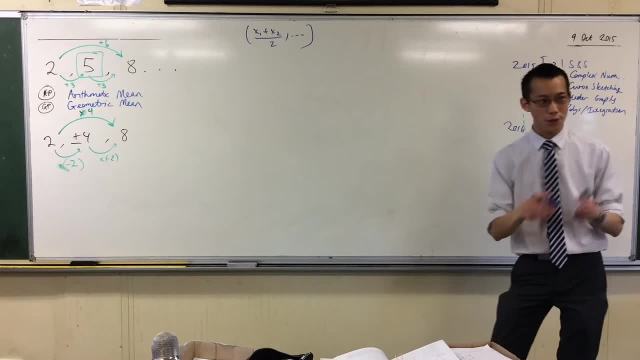 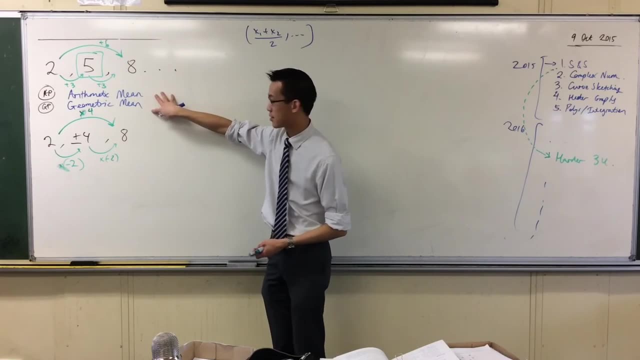 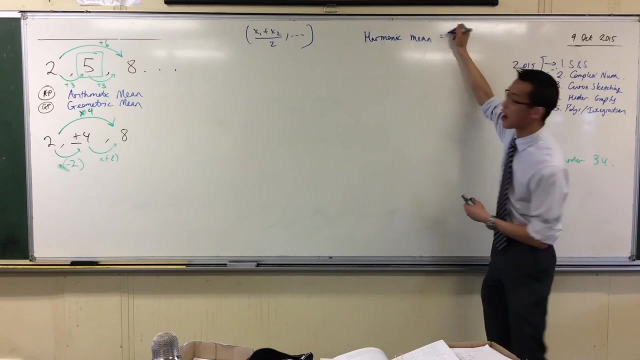 Now I'll let you. I'll leave it for your thought as to why on earth you would want like: in what context would an arithmetic mean or a geometric mean make more sense? There are lots more. I will just tease for you. one of the most interesting means that I think I know about is called the harmonic mean. 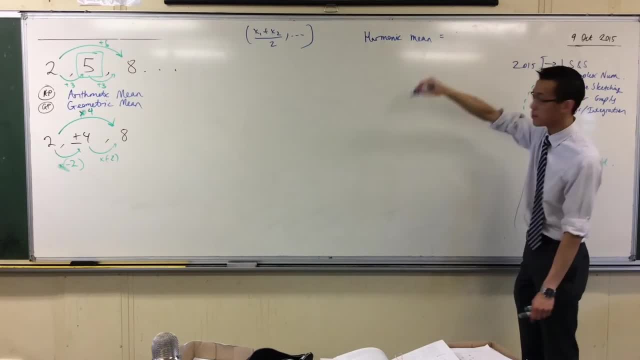 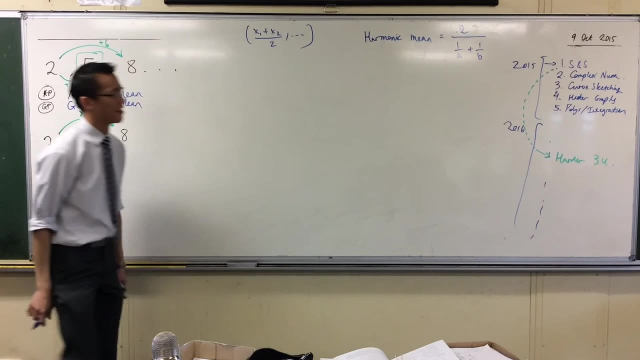 I'm just thinking about two numbers here. The harmonic mean is if you've got two numbers, you get two divided by the reciprocals of the two numbers right Added together. That looks really weird. What on earth could that be useful for? 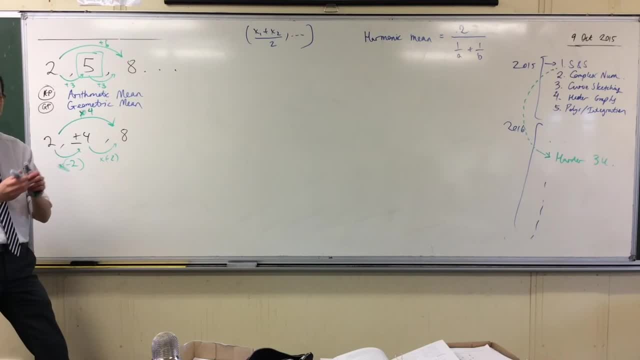 I'll let you have a think about it. okay, I'll, I'll, I'll give you a bit more of a clue at the end, but I'm not going to come out and tell you, because it's more interesting if you try and find it yourself. 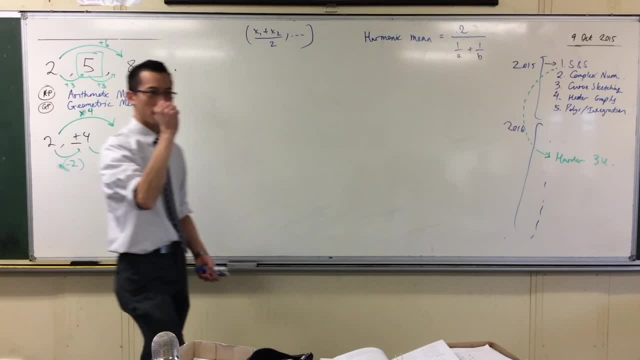 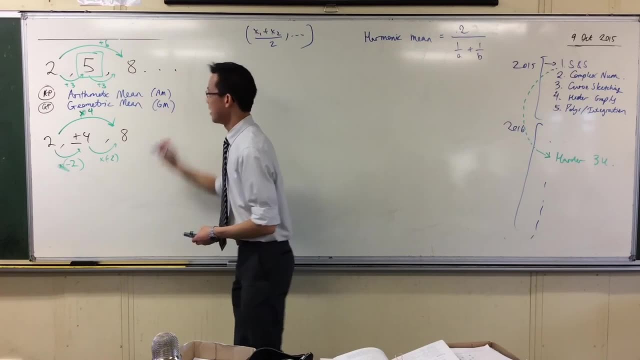 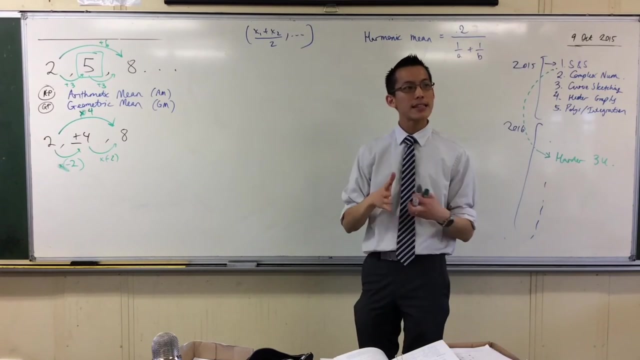 Okay, So these two numbers here right? The arithmetic mean, also known as the- everything gets abbreviated in this topic- the AM- and the geometric mean the GM. okay, It's not hard to find when you've just got actual numbers. right Now let's think abstract. 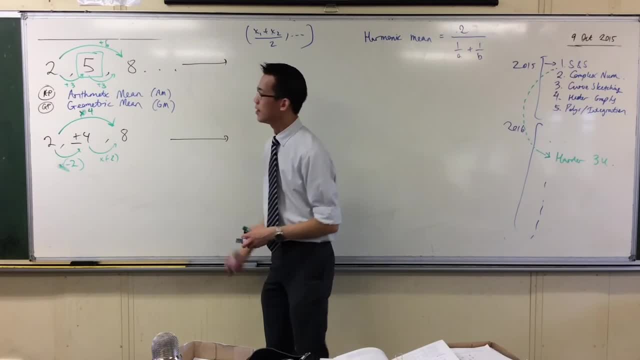 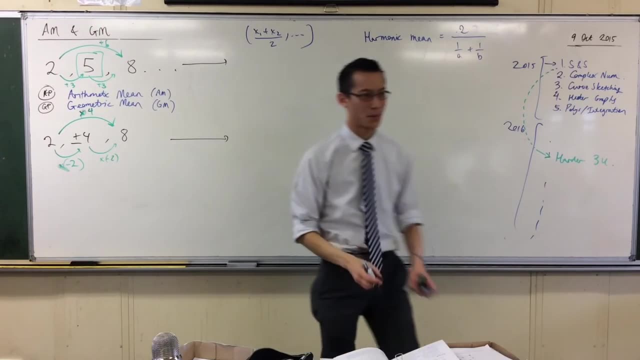 Okay, let's think abstract. So now I'm going to go over here. Oh, and, by the way, that was kind of your kind of your heading AM and GM. I'm so lazy I'm not even going to write the proper words. 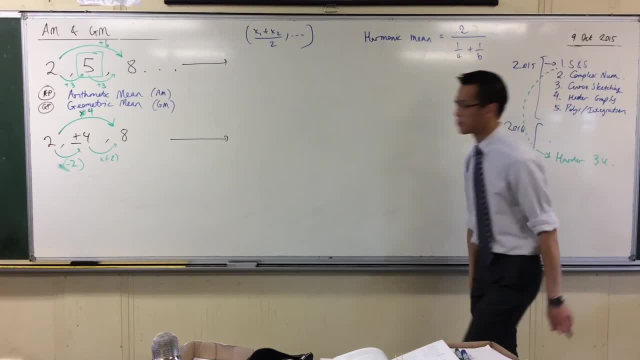 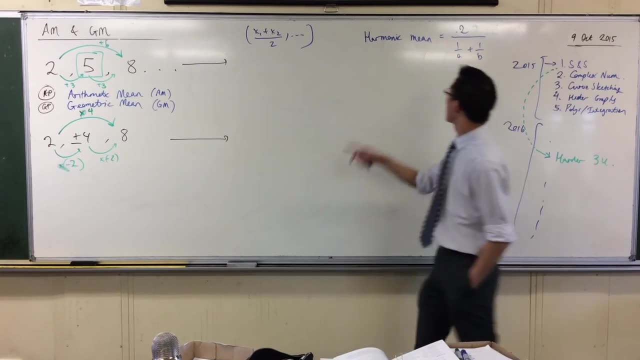 Now I want to think algebraically, because I'm not always going to get 2 and 8, am I? I'm going to get all kinds of different things right. So if I have two numbers and I'm going to call them A and B, okay, A and B. 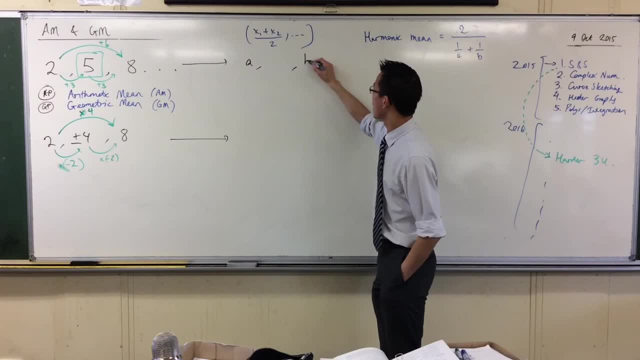 I've got A comma something and then B, I literally have on the board. what am I going to do to those two numbers? in what way can I combine them in order to get this number in the middle for an AP? 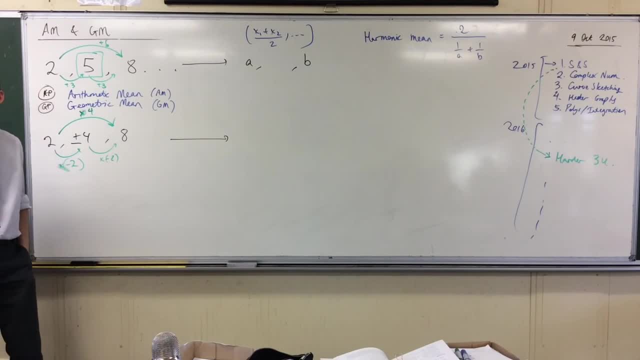 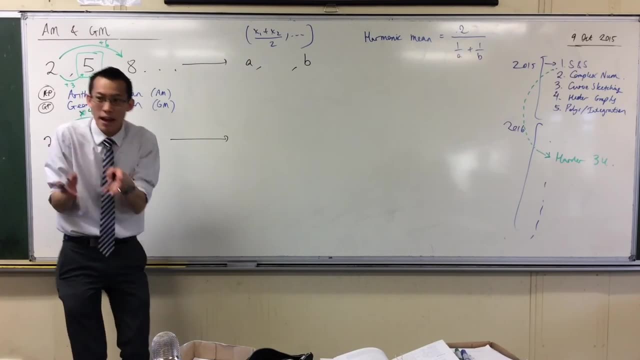 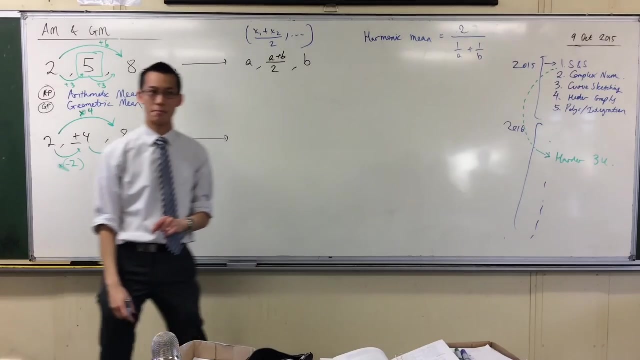 Can you see? It's literally actually right there above me. I want to take the arithmetic mean, the average, right? That's the average we're familiar with. okay? So that's just: you add those numbers together and divide, okay, Divide by 2.. Are you happy with that? 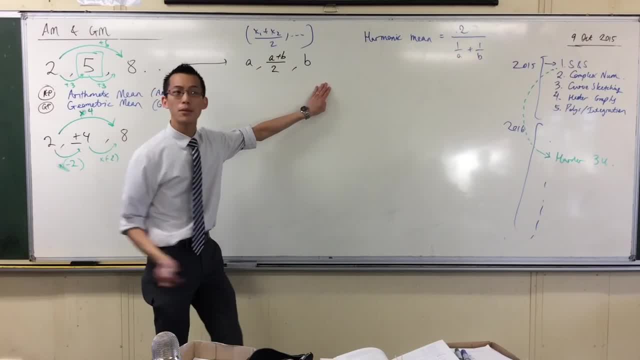 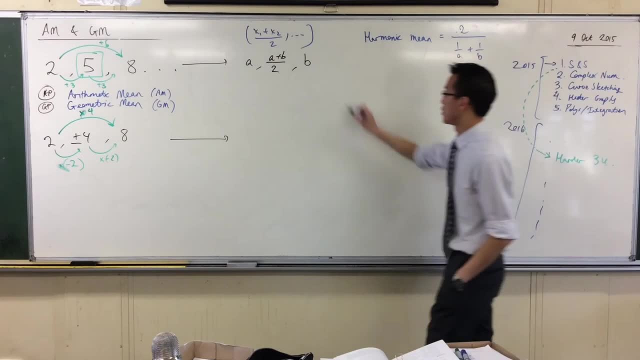 This will always be an AP. You can put any numbers you like in there. They can be positive, negative. anything is going to work, And our 2,, 5, 8 example proves it. Dot, dot, dot. This is our. 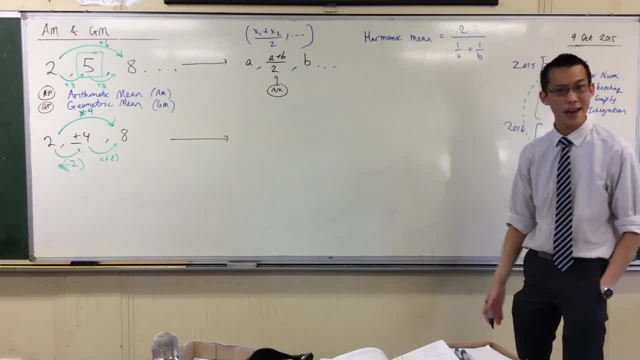 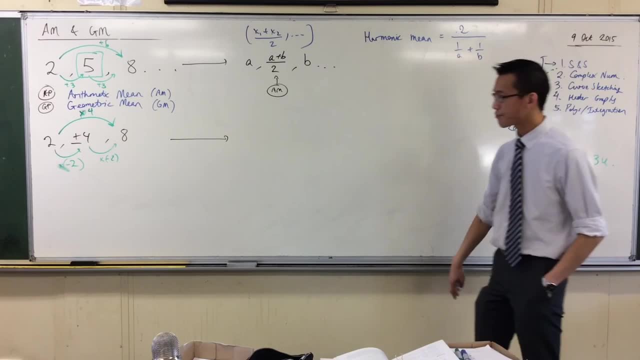 formula for the AM. okay, That's our formula, Just like we had a formula for the nth term and we had a formula for we're going to get quite a few formulas in here. That's the one for the AM. Okay, now think this one's a little more tricky, right? 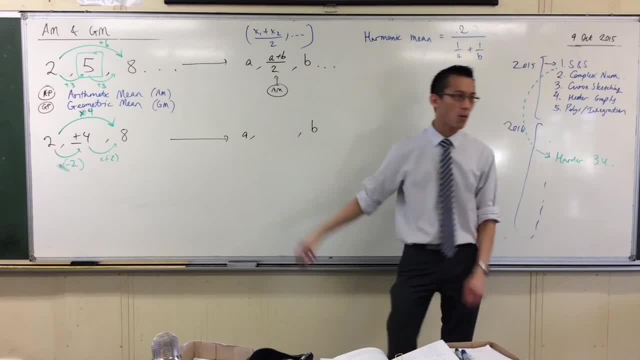 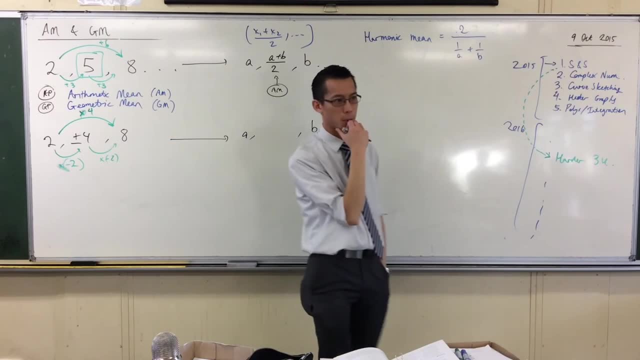 If I still have A and B, but I want the GM now Think about the process we went through to get this and how it compares to this. Hmm, how did we end up with 4?? More specifically, plus or minus 4?? 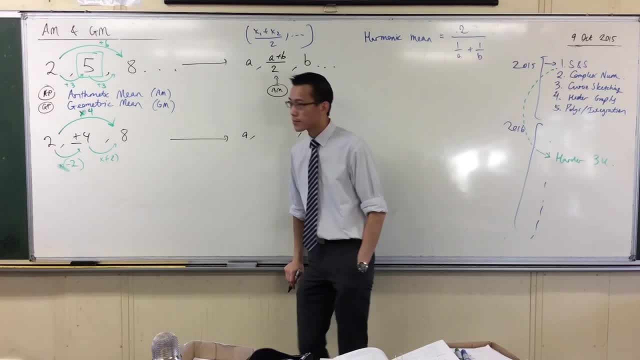 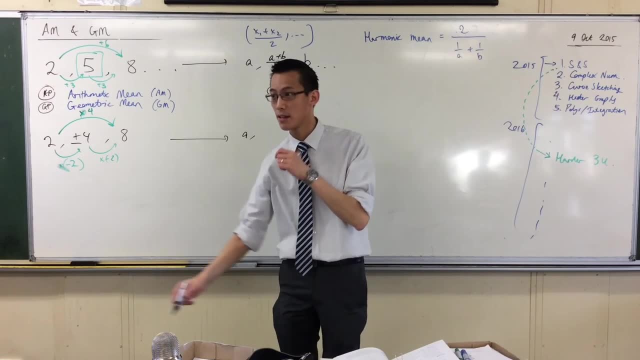 It's actually a clue, by the way. Yeah, Raph. Um, it's the square, it's the Yeah. yeah, yeah, you're on the right track. Just pause for a second before you go on and finish your thought. 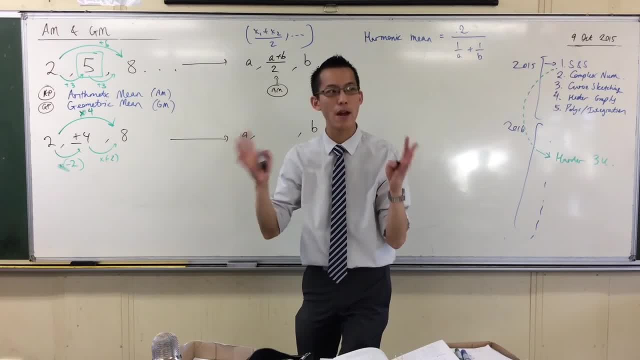 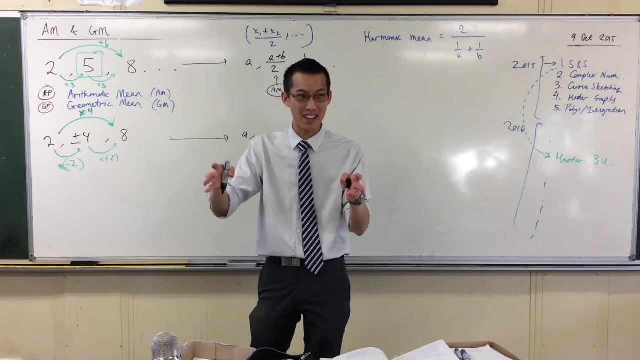 All of you should be thinking, you should be suspicious and think a square root's got to do with it somehow, because where else do we get plus or minuses coming up right? It's when you take the square root of both sides of something and you need to have both, okay. 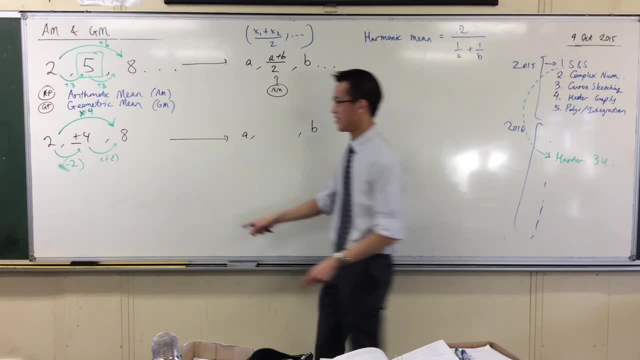 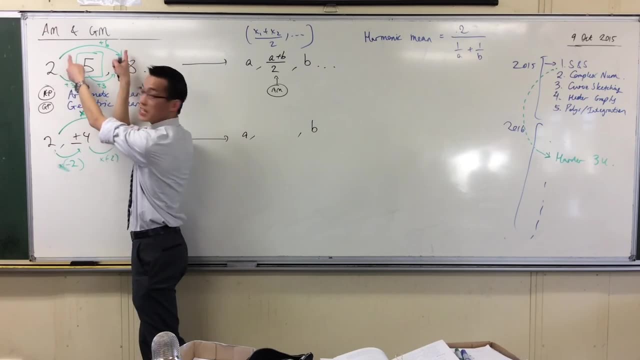 You want to try and finish your thought. The square root of the first term times the third term. Okay, yeah, we got the numbers right this time, right, So you have a look here. right? I combine the first and third terms by addition here because it's an AP. 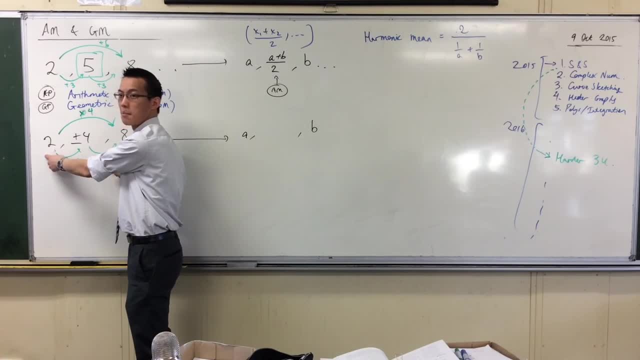 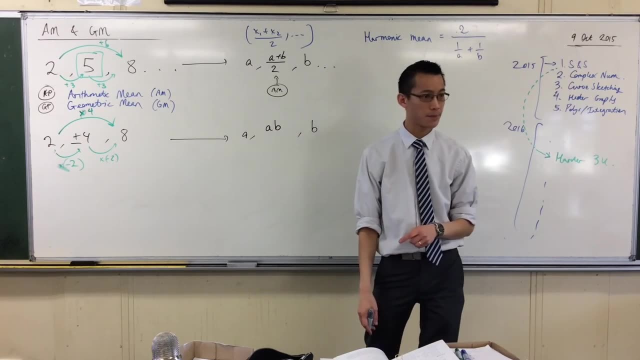 But I want to combine the first and third terms here by multiplication, because it's a GP. You're getting this right. So in the middle here, what I start off doing is I take the product right And you can see when I do a 2 by 8, you're getting 16.. 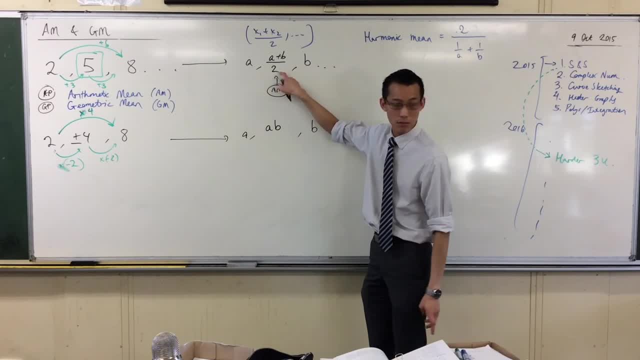 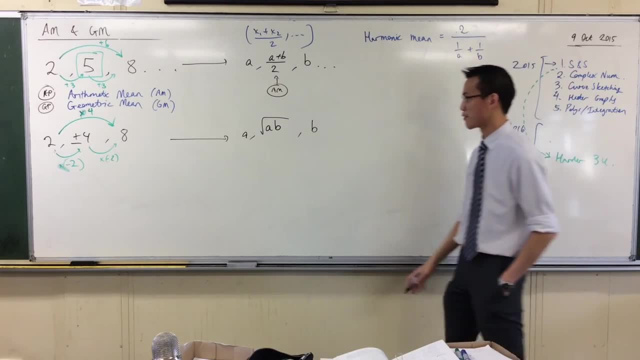 So, to come back to the middle, instead of dividing by 2, you're going to take the. Why did I write that so hard? You're going to take the square root. okay, Now, as we have noticed. Thank you, Brendan, okay. 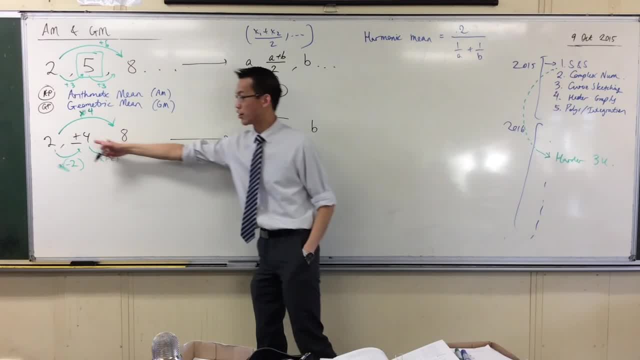 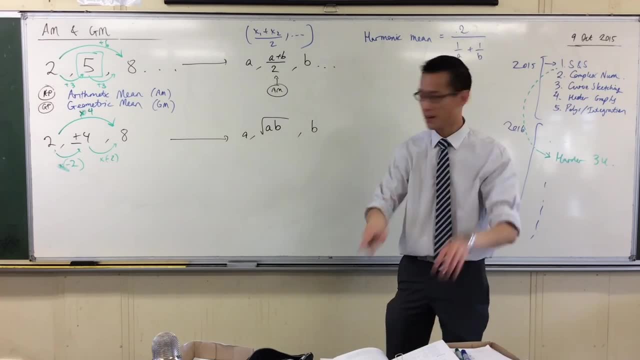 This is not the only option for the GM. You can get the plus or minus. We saw in our first lesson on GPs that you can get that alternating thing. Remember that Black green, black green, black green. So I can do plus or minus in here and they're both fine okay. 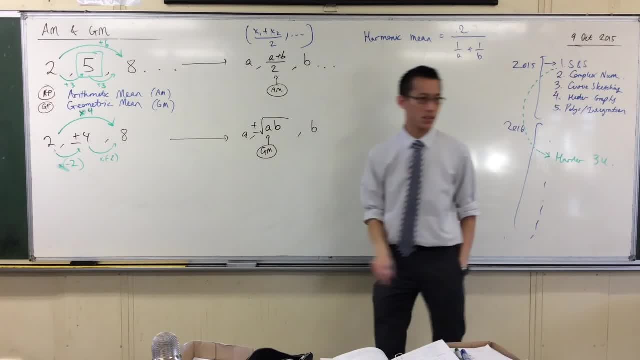 This is our formula for the GM. okay, So I'm going to take one and have to get a plus there with a negative, Yeah, and you're going to find in your End: VND, what's totally really attractive about being at random and being 선생님. something that really you don't want to think of, Like, oh, I shot my GM to be negative tomorrow because he's left behind And you don't do that. So if you're in a place that Lightning has a positive, then you're going to have to go. hemat Wirtschaft. between two of your GPs okay.